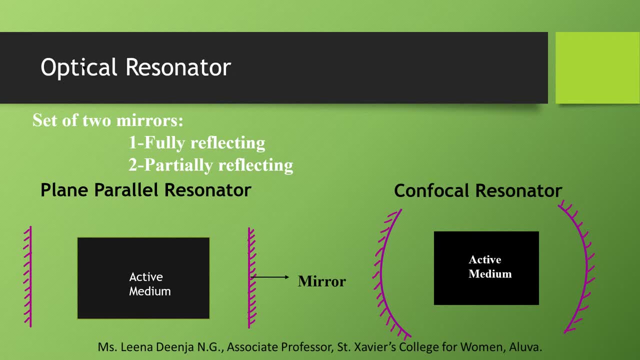 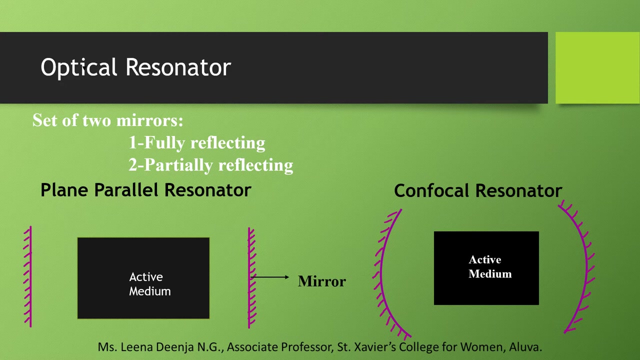 For this we can use a pair of mirrors, with one fully reflecting and another partially reflecting. Such pair of mirrors that is used for light feedback in lasers is known as optical resonator or optical cavity. Active medium is always placed between the mirrors. If the mirrors used are plain, it is called a plain parallel resonator. 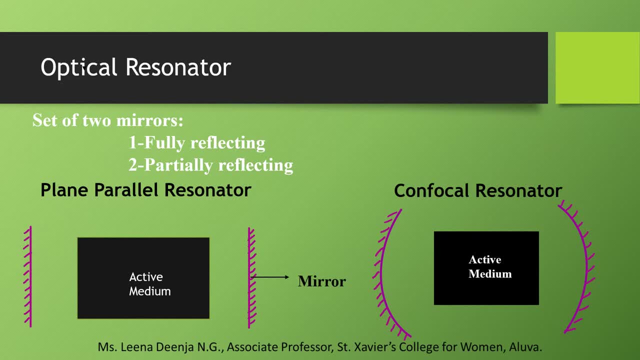 A plain parallel resonator is a medium that is used for light feedback in lasers. A plain parallel resonator consists of a pair of plain mirrors facing each other. A confocal resonator system consists of a pair of mirrors of equal radii of curvatures, separated by a distance equal to the radius of curvature. 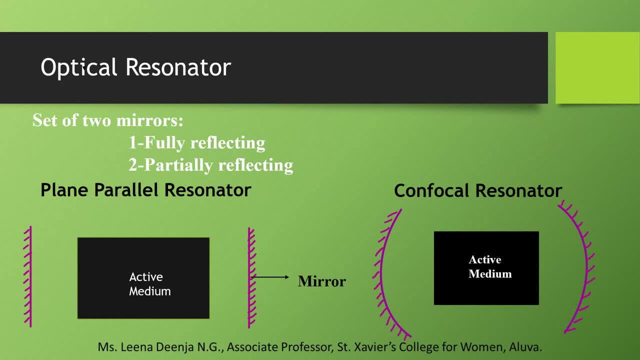 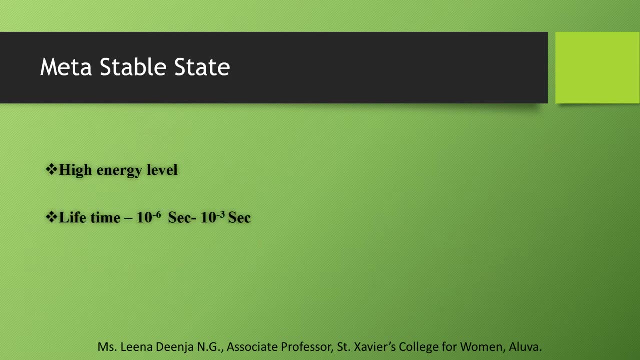 The active medium is kept inside the concave mirror. symmetrically, Atoms or molecule can stay for any duration In lower energy state or ground energy level. but when the atoms absorb energy from pump source, they will jump from lower energy level to upper energy level. 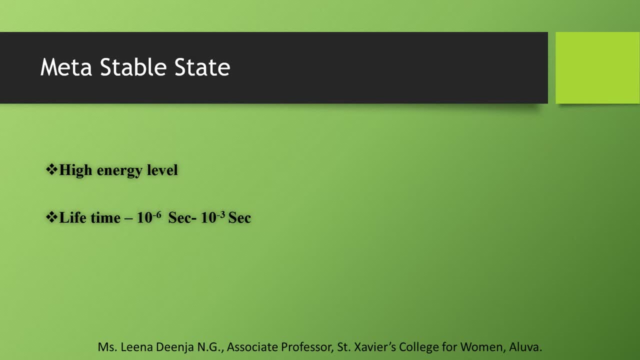 Normal life time of the upper energy level is about ten raise to minus eight seconds. So suddenly atoms released their energy through spontaneous emission. For laser emission, accumulation of atoms in higher energy level and in thefレ and subanyi emissi, silent energy situation. 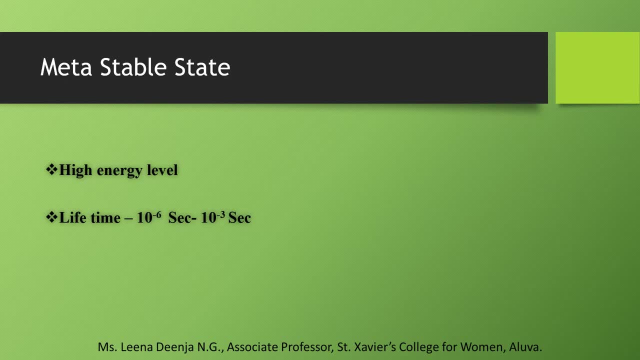 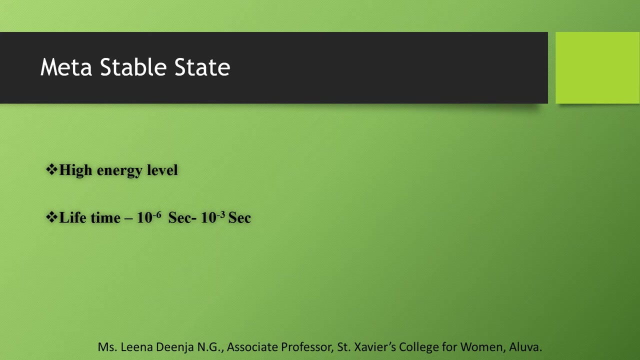 and thereby population inversion is needed. This is possible only when lifetime of the upper energy level is high. Such a high energy level, with lifetime of the order 10 raised to minus 6 second to 10 raised to minus 3 second, is called metastable state. 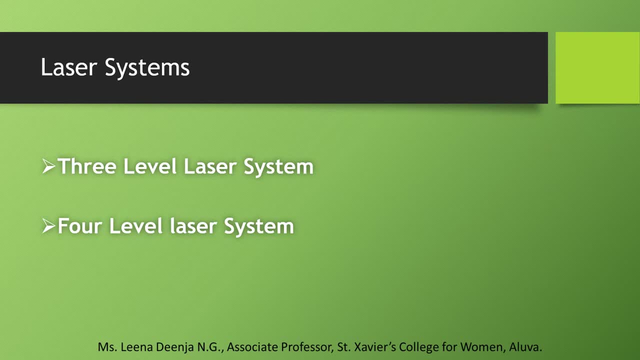 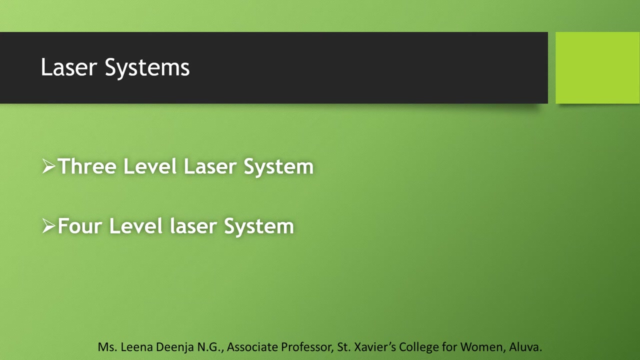 Atoms in general are characterized by a large number of energy levels. Depending upon the upper and lower laser level, laser systems are classified into 3-level and 4-level laser system. Now let us discuss what is meant by a 3-level laser system. 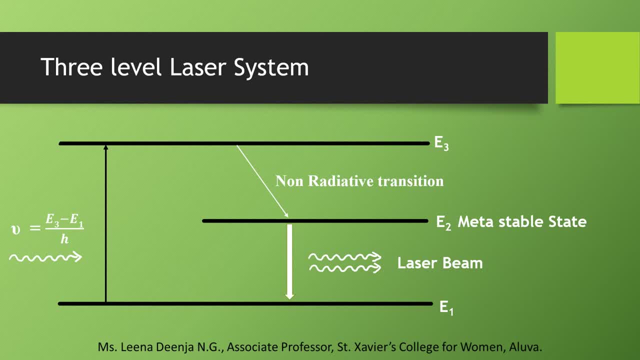 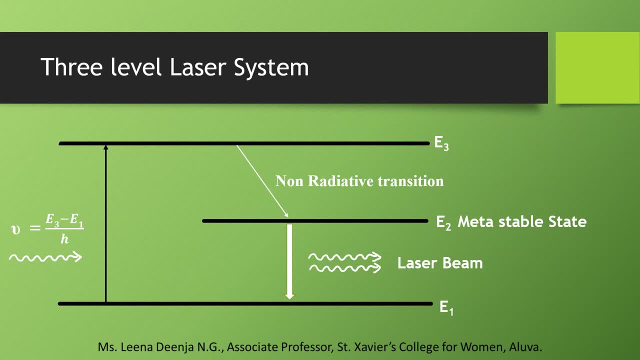 Here the energy levels of atoms are E1, E2, E3, etc. Since atoms in lower energy level is more stable compared to that in upper energy level, normally most of the atoms are in ground energy level, E1.. Suppose the medium is irradiated or pumped with suitable frequency. nu equal to E3-E1 divided by h. 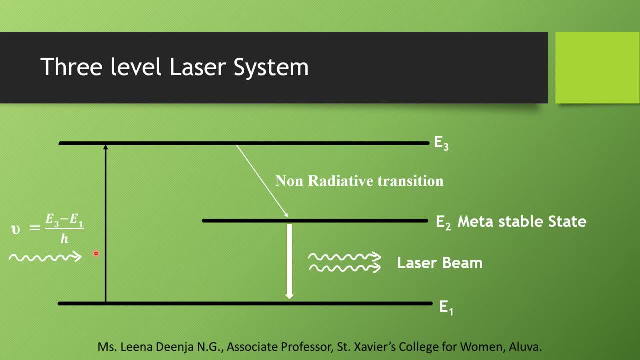 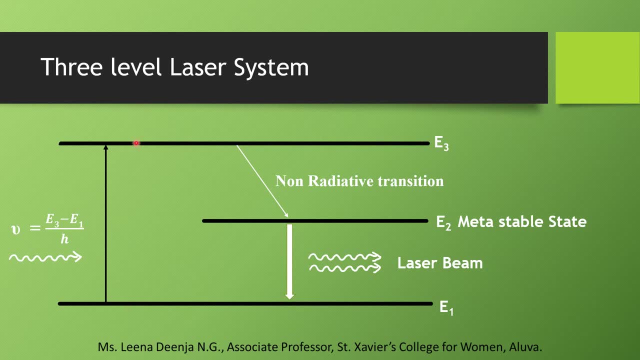 Atoms in ground energy level will absorb this frequency and will jump into higher energy level E3. But for this higher energy level lifetime is of the order 10, raised to minus 8 seconds. So atoms cannot stay in this level for long time. 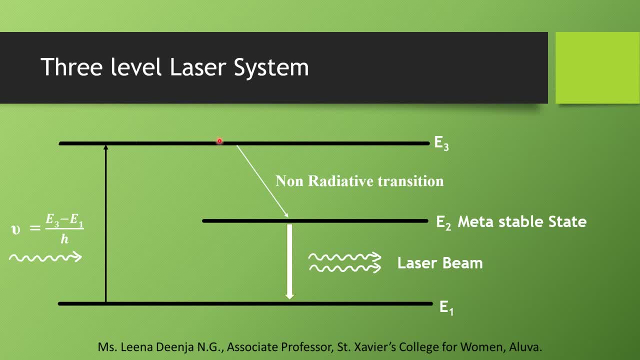 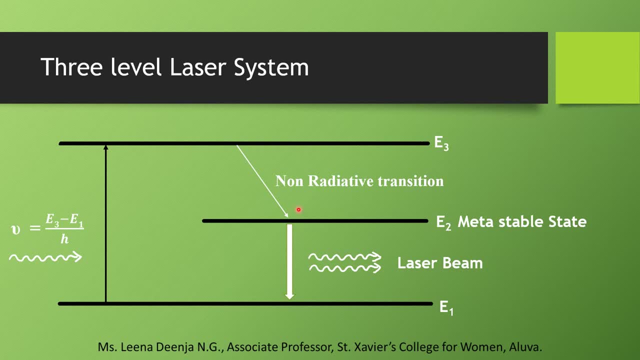 So suddenly it will jump to next lower energy level, E2. And here this jump. it is actually a non-radiative transition. If E2 is a metastable state, its lifetime will be about 10 raised to minus 6 seconds to 10 raised to minus 3 seconds. 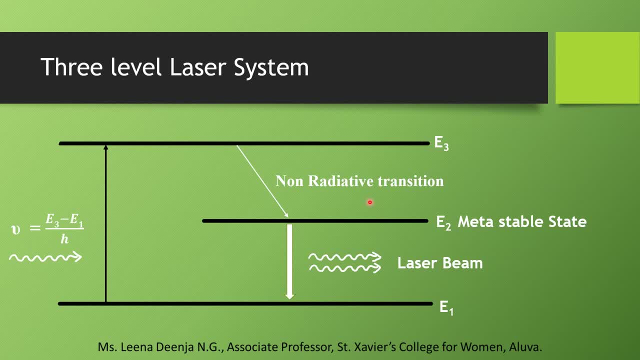 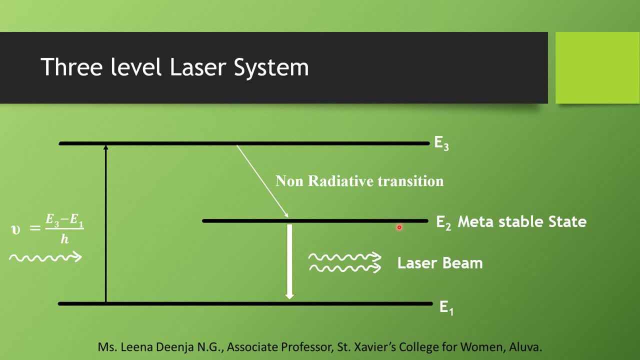 So atoms can stay for more time in this metastable state. When pumping continues, accumulation of atoms in this E2 level increases. After a short interval of time when more than half of the total total atoms accumulate in this E2 level. 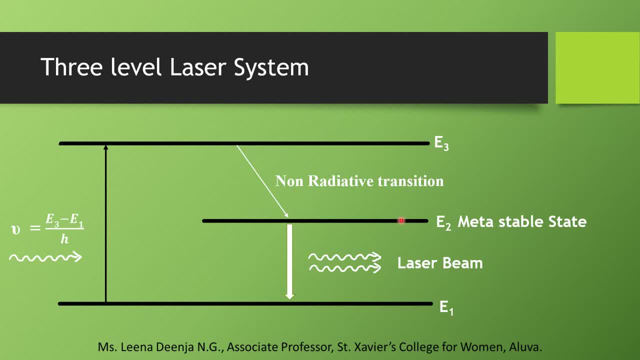 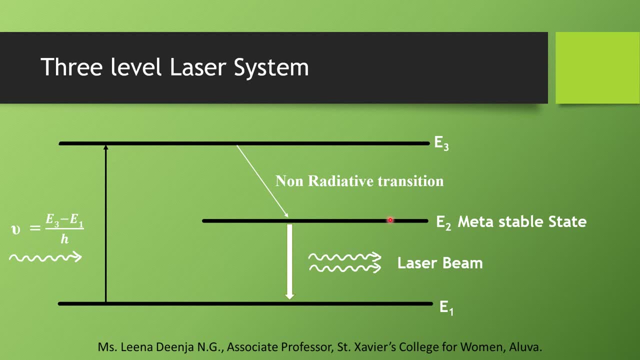 there is population inversion set up between this E1 level and E2 level. Now it is ready for laser action. A spontaneously emitted photon can trigger stimulated emission which results in laser emission. Here the laser emission is between one of the higher energy level, E2,. 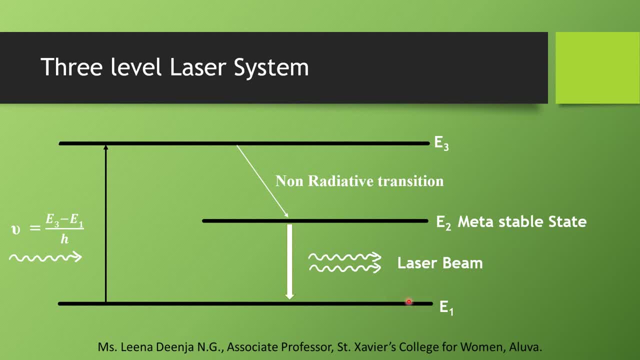 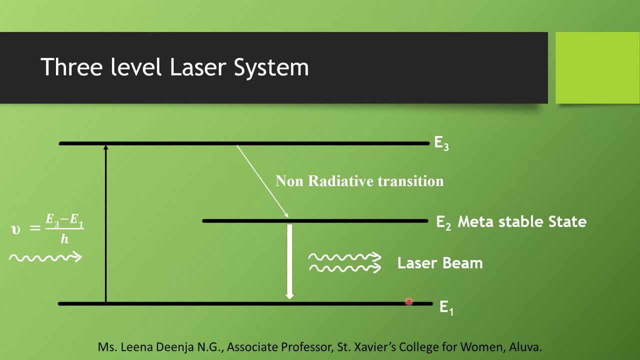 and lower energy level. E1. This means upper laser level is one of the higher energy level and lower laser level is ground energy level. Such laser systems are known as three-level laser systems. After laser emission, all the atoms are in lower energy level. 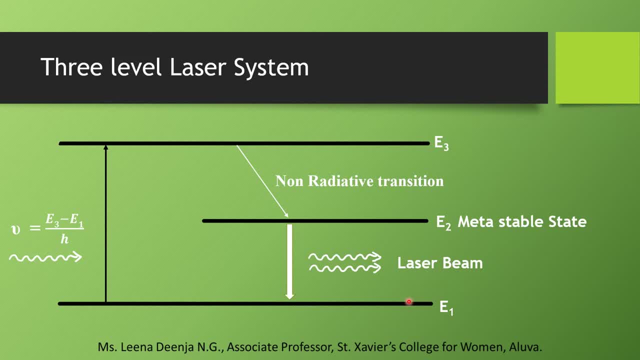 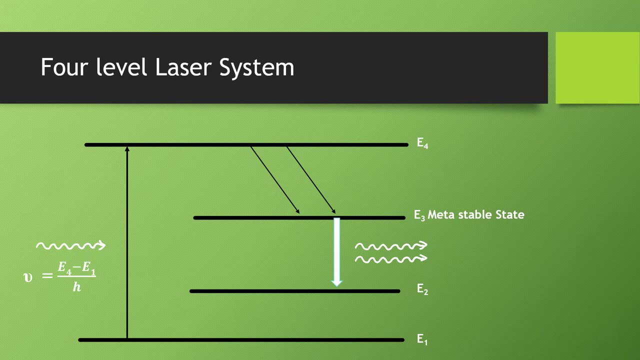 Now the system has to wait for another population inversion for laser action. So here the laser output is pulsed. Now let us discuss what is meant by a four-level laser system. Here the energy levels of the atoms are E1, E2, E3, E4, etc. 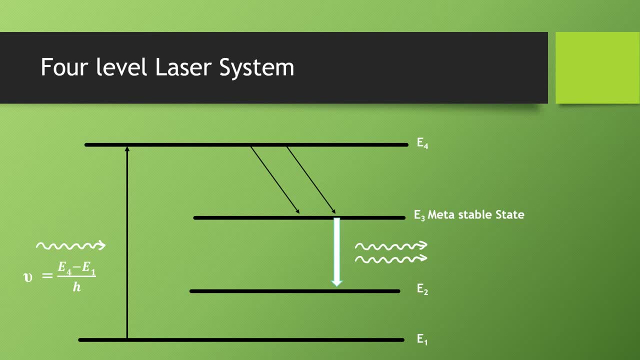 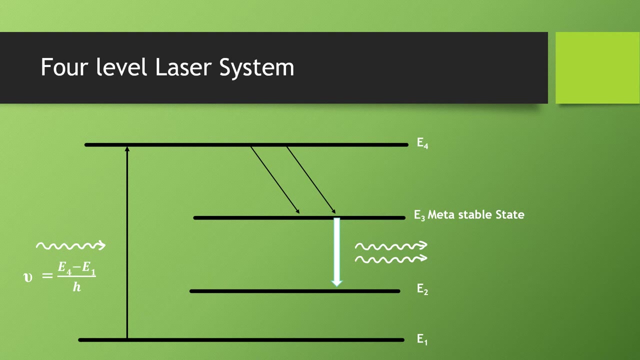 Due to the stability, most of the atoms prefer ground energy level. When the medium is irradiated with pump frequency nu equal to E4-E1 by h, many atoms from ground state will be excited to go to the pumping level E4.. 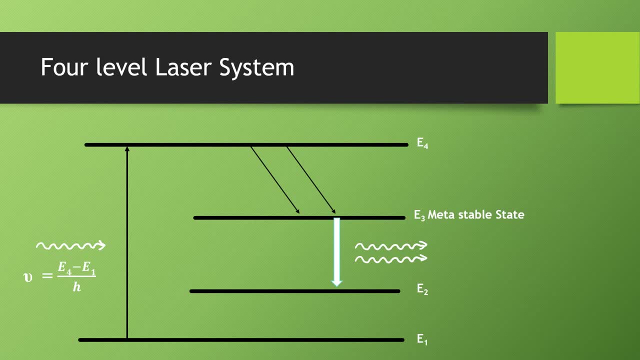 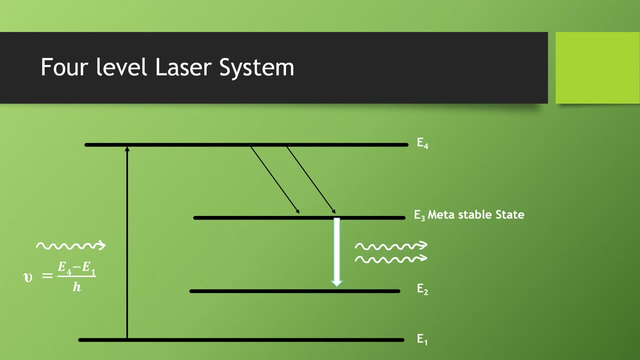 Since lifetime in this E4 level is very short of the order of 10 raise to minus 8 second. atom makes non-radiative transition from E4 to meta stable state, E3.. For E3 level, lifetime is about 10 raise to minus 6 second. 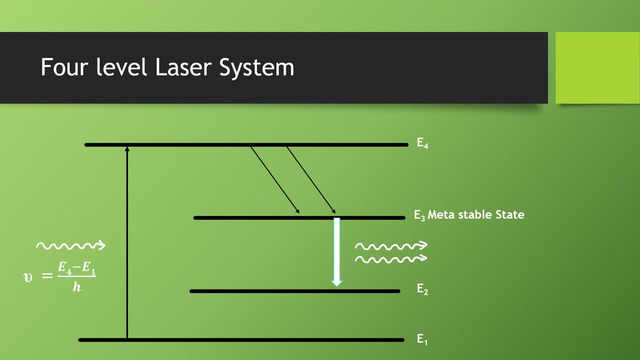 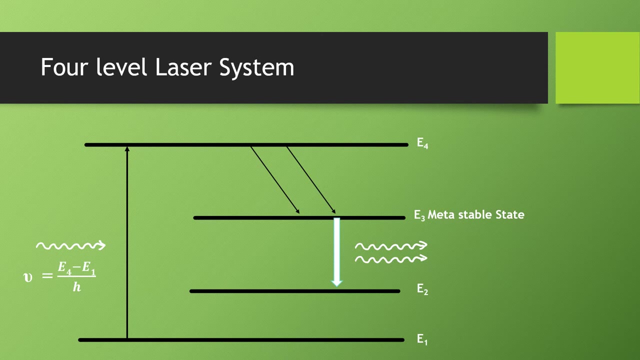 6 second to 10, raise to minus 3 second, So atoms can stay for more time here. Just below E3 there is another energy level, E2, which is unpopulated. As time passes and pumping continues, there is always population inversion between E3 level and E2 level. A spontaneously emitted photon. 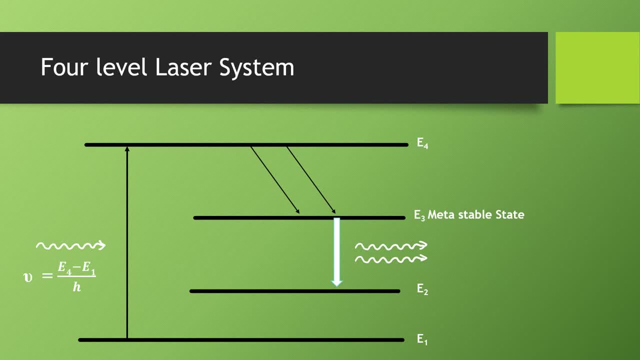 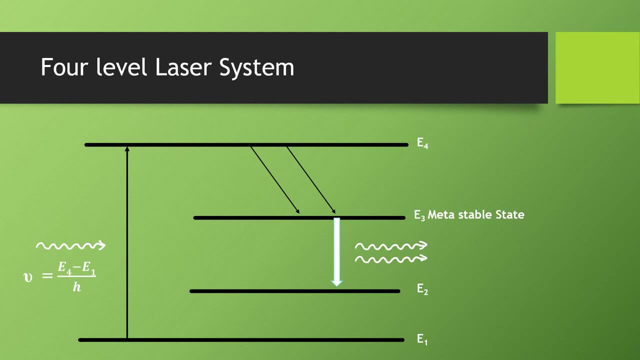 of energy, h nu, which is equal to E3 minus E2, can trigger laser action here. Once the atoms reach E2 level they will undergo non-radiative transition and will jump to ground energy level. So here there is no need to excite more than 50 percentage of atoms in ground state to upper level. 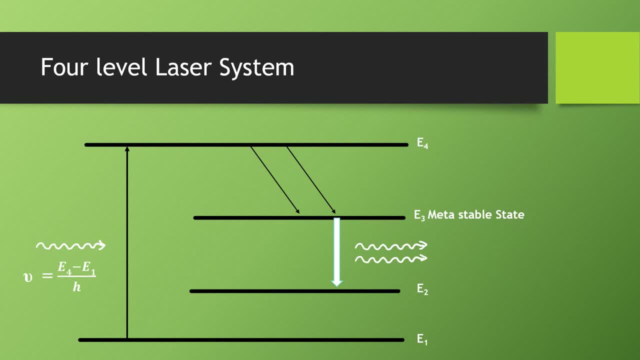 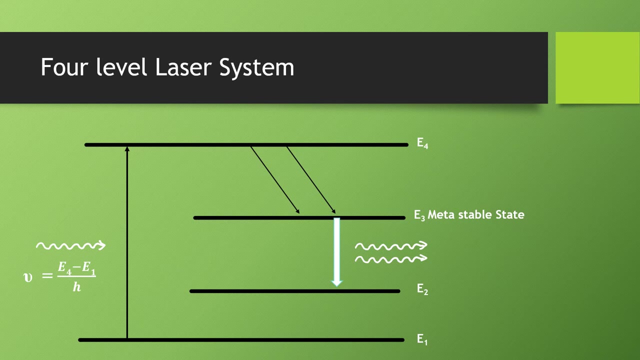 for population inversion. Here the laser action takes place between two higher energy levels, E3 and E2.. E3 is upper laser level and E2 lower laser level Due to continuous population inversion between E3 and E2. the laser emission is always continuous Laser transition due to population inversion between